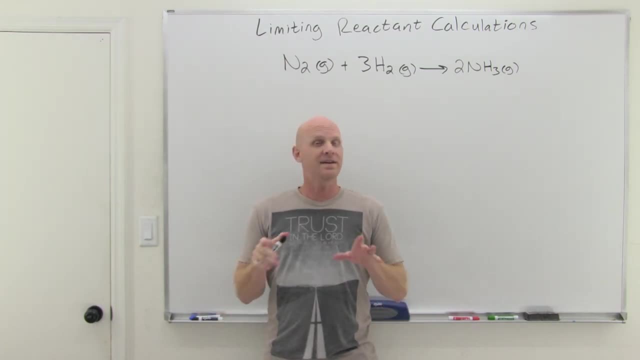 tanks sitting on the side of my house, And so you should have said: I don't know, And the key is this, and the big point I'm trying to make, I'm being a little bit, you know, tongue-in-cheek. 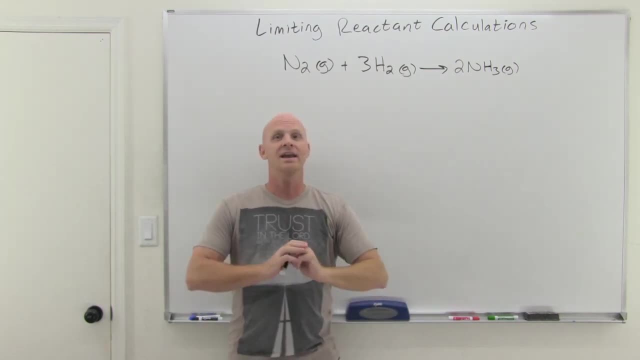 here. but the big point I'm trying to make is that a balanced chemical reaction never tells you what you have. So I don't know. I don't know what you have. I don't know what you have, I don't know what. 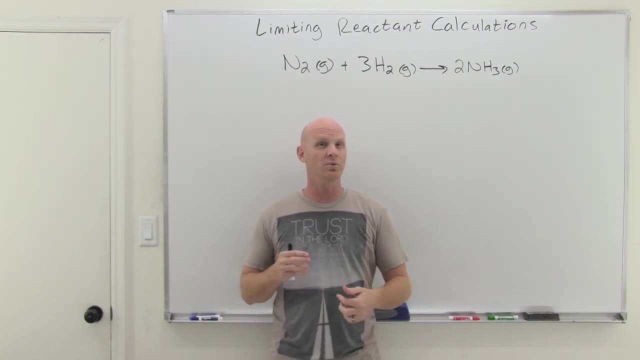 you have. It never tells you what you have. It is only going to tell you the mole-to-mole ratio in which things react. So in this case it says that one mole of N2 gas reacts with three moles of H2 gas to produce two moles of NH3 gas. It's a one to three to two ratio, And that is all it. 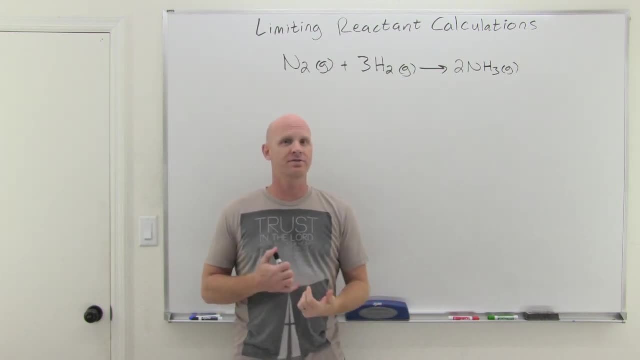 tells us. So how much we actually have of either of these reactants or products is something that's extraneous, that has to be given. So if I told you that I actually do have one mole of N2 gas, I might say, well, 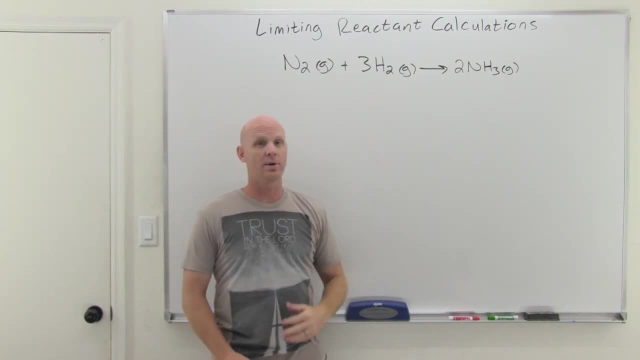 do I need to react with it? Well, based on the one to three ratio, I would need three. What if I said I have two moles of N2 gas? Well then, how many moles of H2 gas would I need for it to react? 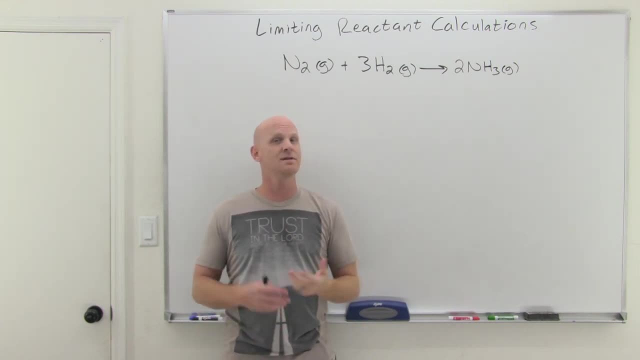 with. Well, we'd say six, because that two to six ratio reduces down to that one to three ratio. And so again, your coefficients here, ultimately, are only going to give you a new way of finding mole-to-mole ratios, a one to three ratio, if you're comparing N2 to H2.. Or if you're comparing 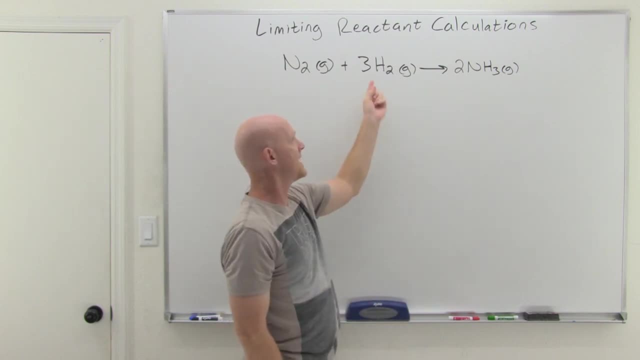 N2 to NH3, it'd be a one to two ratio. Or if you're comparing H2 to NH3, it'd be a three. So you can compare any two species out of the reactants and products and get a mole-to-mole ratio. 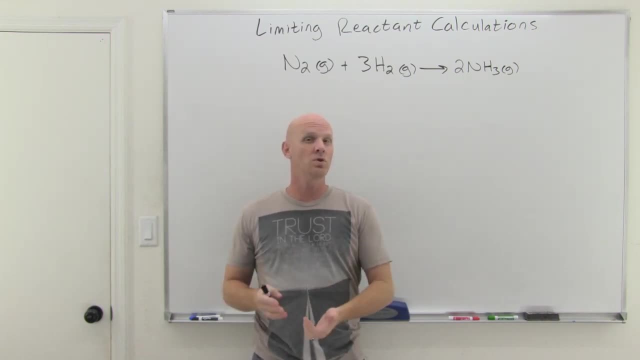 out of that, And so earlier in the chapter we found out that you can get a mole-to-mole ratio from a chemical formula. Well now, and I hinted towards it at the time- you can also get it from the coefficients in a balanced chemical reaction. But again it just tells you the ratios in which. 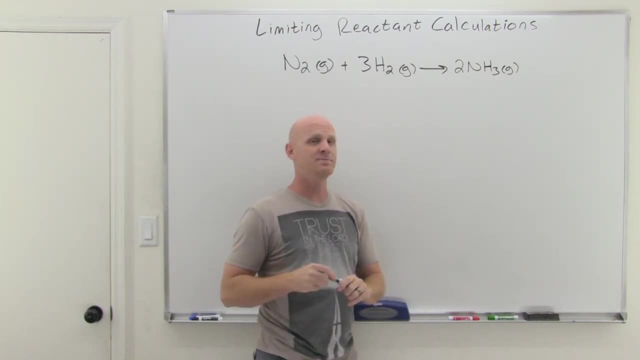 things react. It never tells you what you actually have. That has to be extra information that is provided, And so now I'm going to tell you. So if you've got the study guide in front of you, I'm telling you that to look there. But we've got. 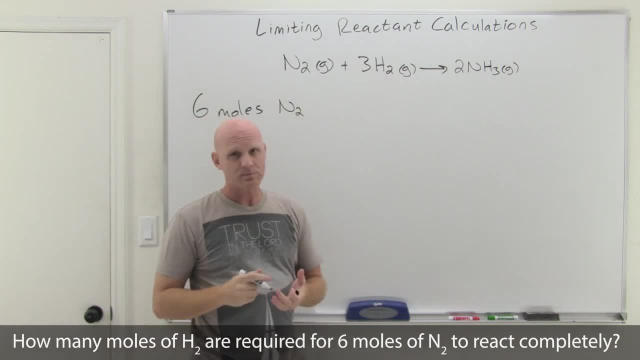 six moles of nitrogen gas And my first question is: how many moles of H2 gas would I need for that to react? that six moles to react completely. And again, the key is based on that one to three ratio And you can probably do this in your head And we're going to do the first few calculations. 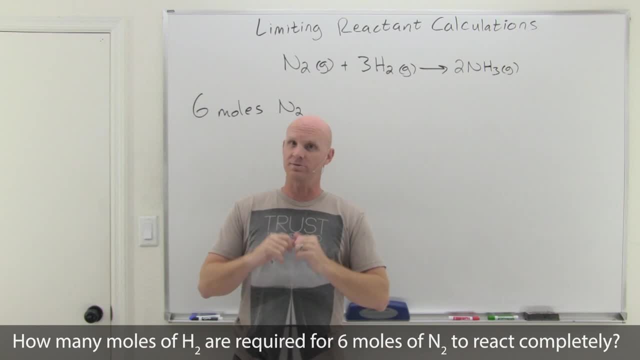 here with numbers that are nice and pretty and things that you might be able to do in your head. In fact, we'll do most of the lesson with stuff that you may be able to avoid using a calculator for, But be prepared, You need to learn this process down pretty good, because you are going. 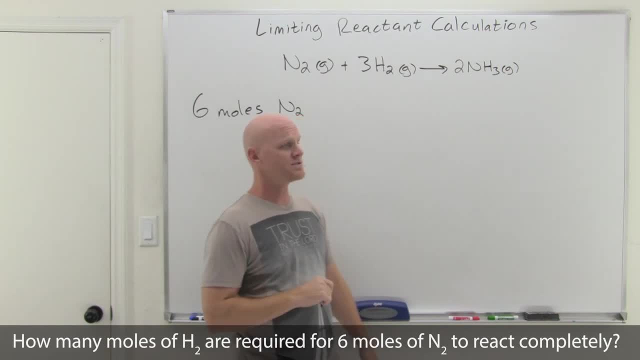 to get problems on your homework and your exams. that will definitely require you to use a calculator, But if we do this without the need for a calculator, it'll make learning the process that much easier. All right, So with six moles of N2, how many moles of H2?? And again based on. 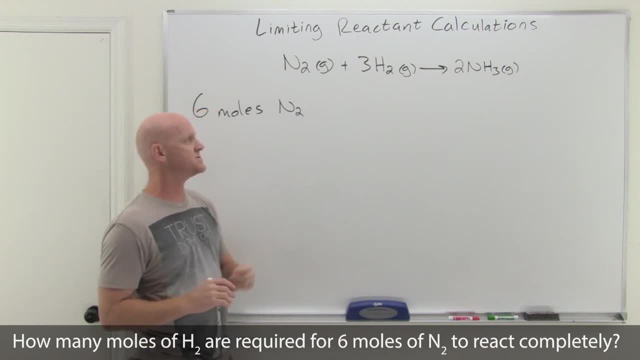 that one to three ratio, I can see it's three times more moles of H2. And three times more moles would be 18 moles of H2.. And that's the answer to this question. Now, if we look at how we work this, 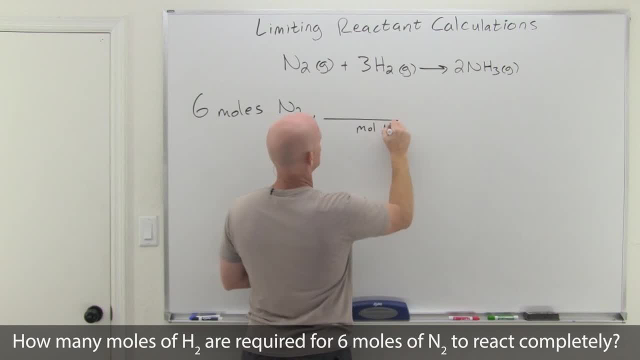 out. what we're going to use here is a mole to mole ratio And we're going to put the moles of N2 in the numerator And for this mole to mole ratio the numbers are just the coefficients in the balanced reaction. So coefficient for H2 is a three And the coefficient for N2 is an implied. 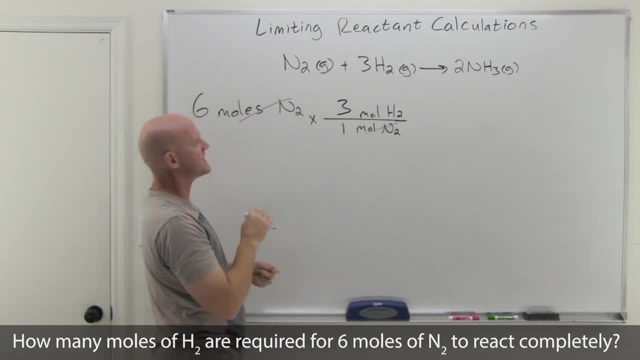 one, And so dimensional analysis gets those moles of N2 to cancel, And six times three over one is indeed 18 moles of H2.. So if I want that six moles of N2 gas to react completely, I would need: 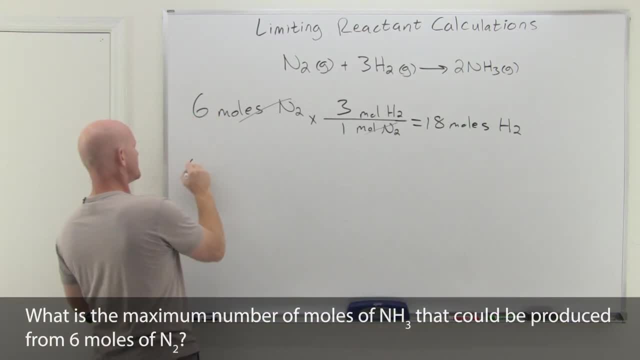 18 moles of H2.. Now, next question: we're going to start with that: six moles of N2 yet again, And this time the question is different. Instead of worrying about how much H2 I need for it to react with, the question is: what is the maximum number of moles of NH3 that can be? 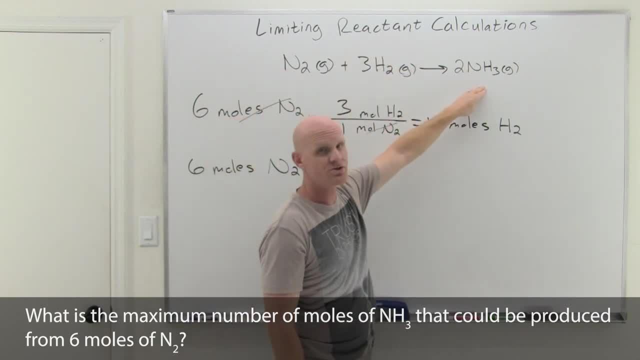 produced. And so in this case I'm relating the moles of N2 to the moles of NH3. And it's a one to two ratio. And so in this case, based on that one to two ratio, you can probably see like well, 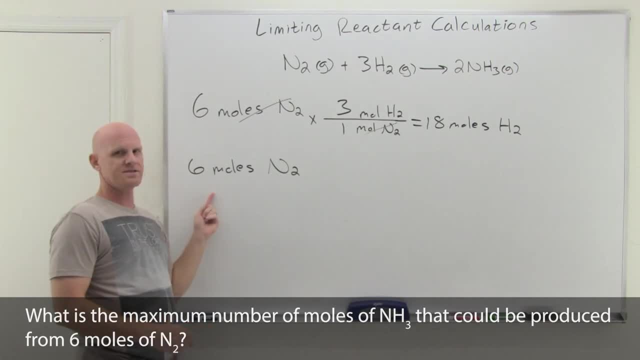 I just get you know, the maximum I get is twice as much, And twice as much would be 12 moles, And that's exactly right. So and again the process, though with the dimensional analysis. here we'll put moles. 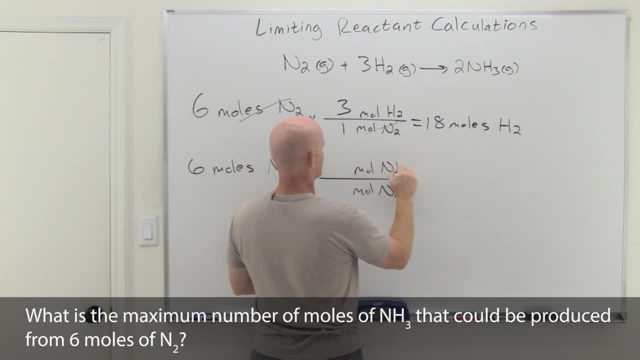 of N2 in the denominator, We'll put moles of NH3 in the numerator. We've got a mole to mole ratio here And again. that mole to mole ratio is just going to come from the coefficients of these two species in the balanced reaction. We get two moles of NH3 for every one mole of N2, according to. 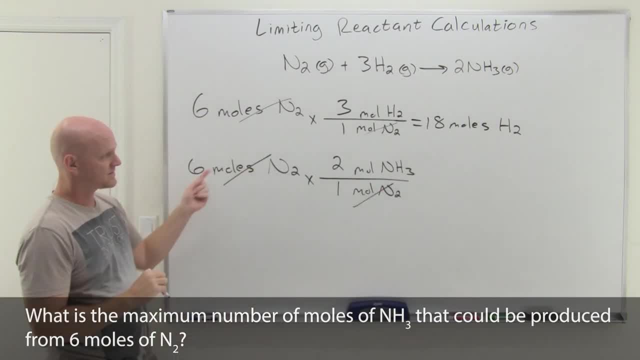 those coefficients Dimensional analysis, those units will cancel. And six times two over one is indeed 12 moles of NH3.. All right, So this is not so bad as long as we're dealing with it entirely at the level of moles. 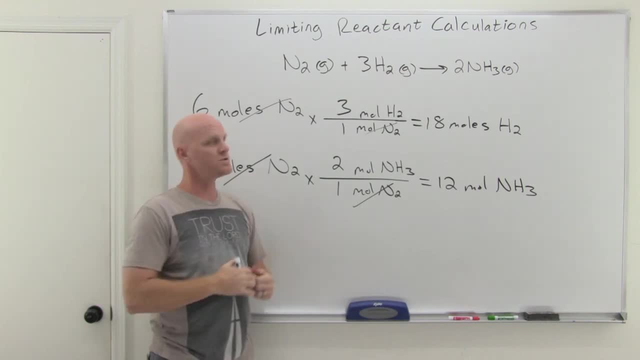 Whether you start with a number of moles of reactant or you're trying to get so many moles of a product or find out how many moles of the other reactants you need. if we stay in the land of exclusively of moles, life is good, It's not so bad And we've got multiple ratios and life is. 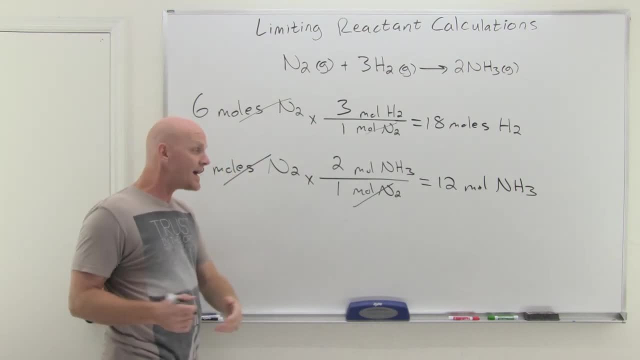 good. The problem comes with what if we start in the land of grams instead? And so, instead of telling you that I've got six- you know six- moles of N2,, what if I told you that I've got 50 moles of N2?? 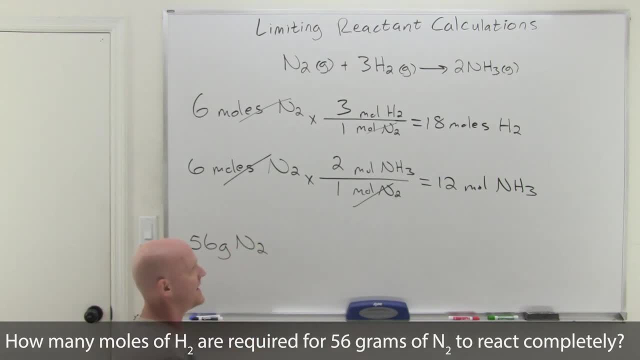 What if I told you that I've got 50 moles of N2?? What if I told you that I've got 50 moles of N2? But I've got 56 grams of N2 instead? And now my question is the same, though: How many moles of? 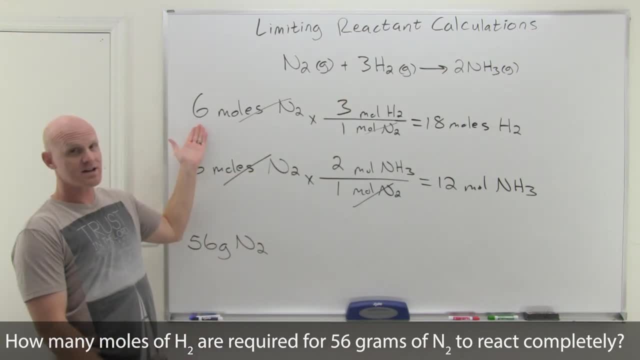 H2 do I need for it to react completely Well? back when we had six moles of N2, when I knew the moles of N2, I just used that three to one ratio to figure out that I needed 18 moles of H2.. And 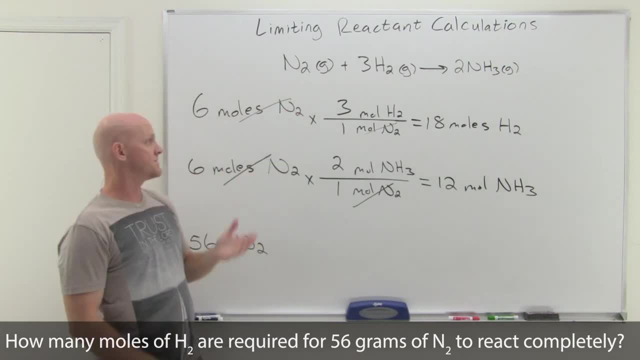 as long as we knew the moles of N2, I just multiplied by that three to one ratio regardless. So if this had been six moles or 10 moles, or a million moles, or 0.437 moles or whatever, 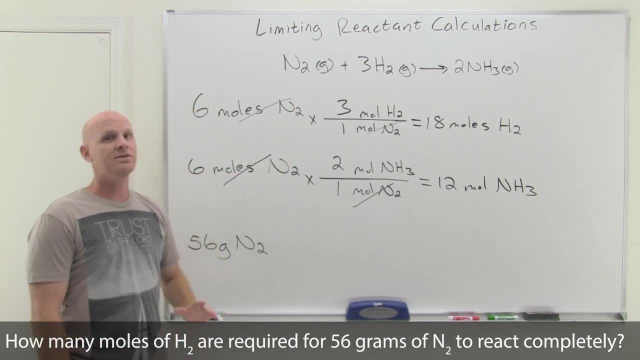 I would have multiplied by a three to one ratio to get there. And so the key is: if you don't know the moles well, then you can't use the mole-to-mole ratio, And so if you're given the grams instead, 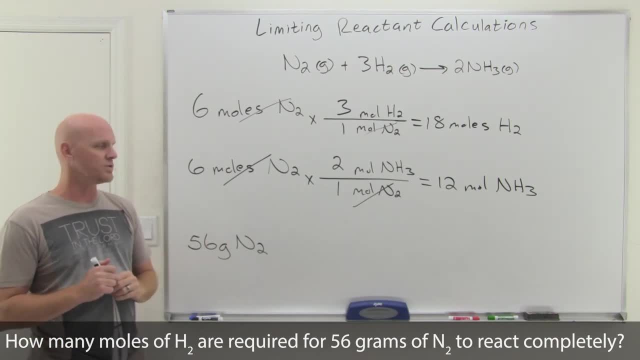 first thing you need to do is convert it to moles, because then you can take advantage of those mole-to-mole ratios. And in this case, how do we convert grams to moles? Well, we'll put grams of N2 in the denominator, We'll put moles of N2 in the numerator, And that connection, if you recall. 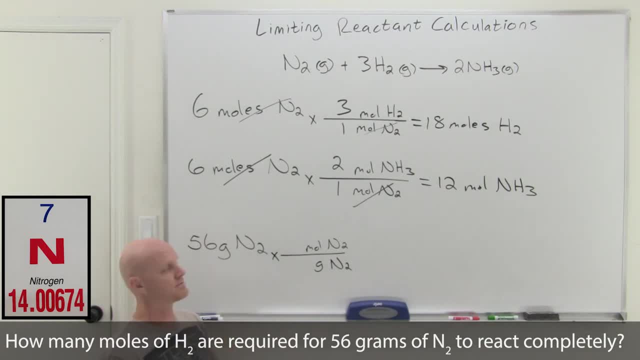 between moles and grams is always, always, always the molar mass. And so if you look at the periodic table, nitrogen has a molar mass, a single nitrogen atom, of 14 grams per mole, But for N2, it's dihydrogenous. So if you look at the periodic table, it's dihydrogenous. So if you 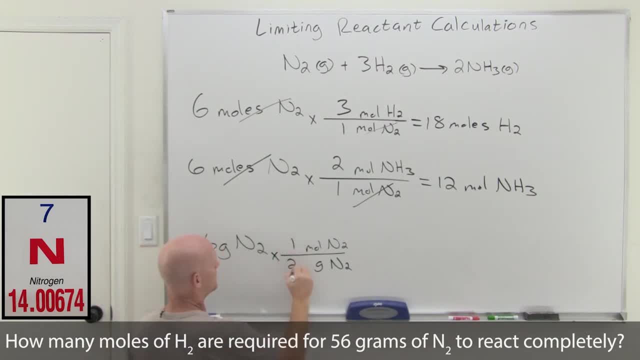 you've got to factor that in, And so it's going to be 28.. And so one mole weighs 28 grams. The grams will cancel, And 56 divided by 28,. I chose this to be nice, So in fact, 56 divided by 28 is: 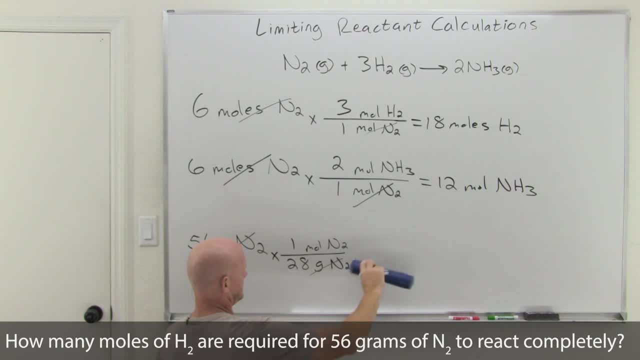 indeed exactly two moles. But let's not stop there And let's not break this up into multiple calculations. We'll then take this a step further And we can now convert it to moles of H2.. We'll divide by moles of N2.. That's our mole-to-mole ratio, And again, that comes from the coefficients. 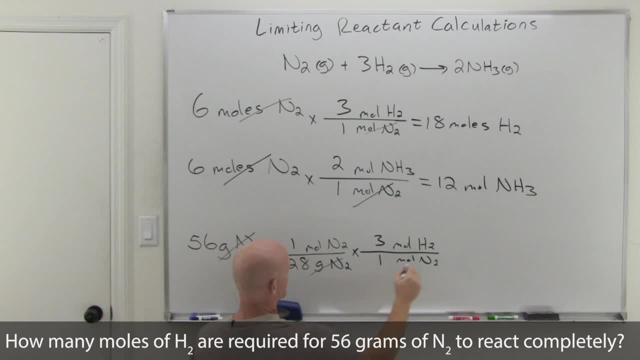 We get three moles of H2 that are required for every one mole of N2 we use up as well. And now 56 divided by 28 is two moles of N2. times that three-to-one ratio means we need six moles. 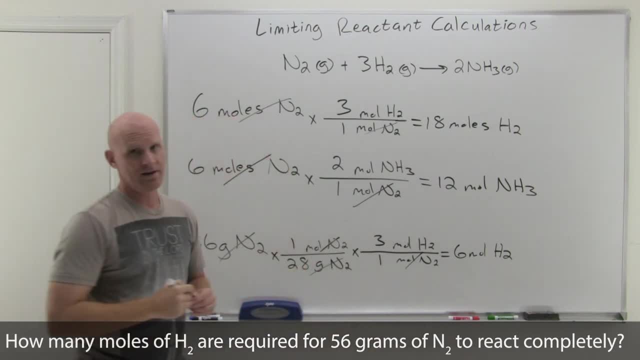 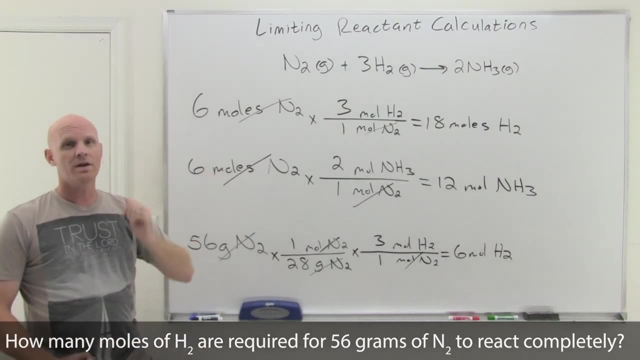 of hydrogen for it to react completely. Now let's just pretend this question had not asked about the number of moles of H2. But let's say I had to take it a step further and it wanted the number of grams of H2.. Well, if we wanted the grams of H2, well then we just need to convert. 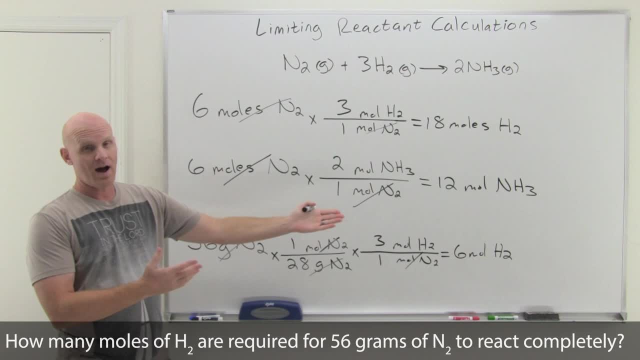 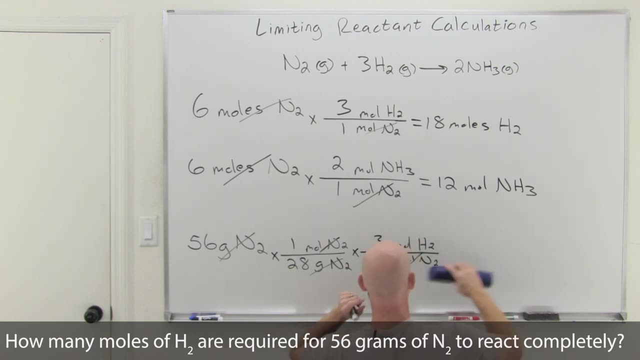 moles to grams at the end, And we could have done that, We could do that, We could do that, But we could have done that as part of the process here And we're going to go back and do that. This was the answer to that question. But had I been asked for the number of grams, we would have just 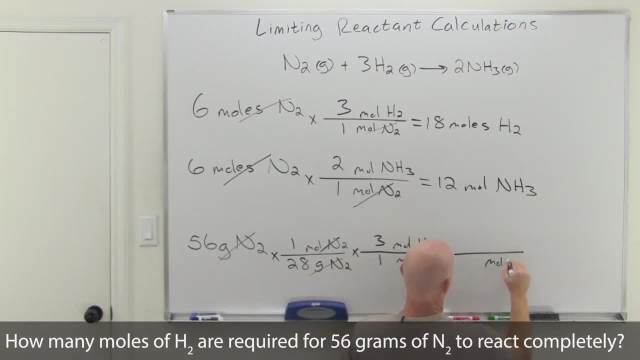 taken this an extra step And to convert from moles of H2 to grams of H2, again, the connection between moles and grams is always the molar mass, And a single hydrogen atom has a molar mass of one gram per mole. But we have H2 diatomic, And so it's going to be one mole weighs two grams. 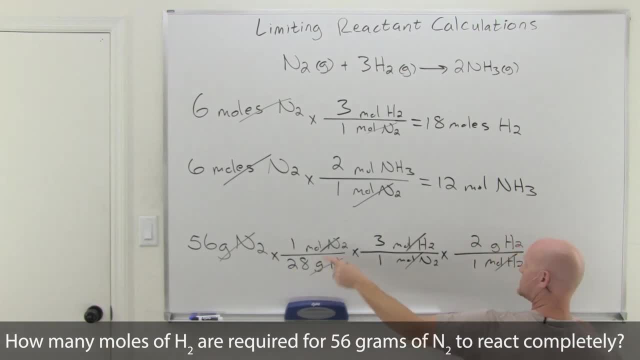 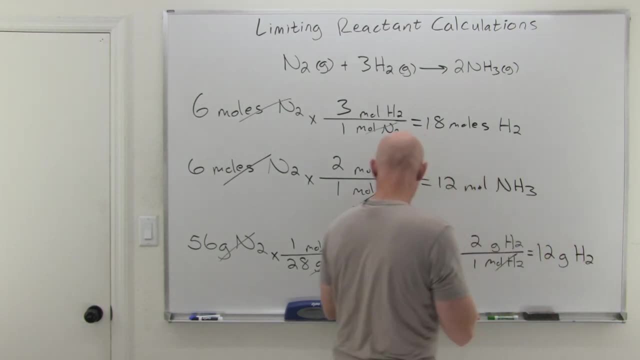 And so in this case we'd get again 56 divided by 20.. It was two Times three is six moles, And times two gets us 12 grams of H2.. This is often when you take it this far, when you start with. 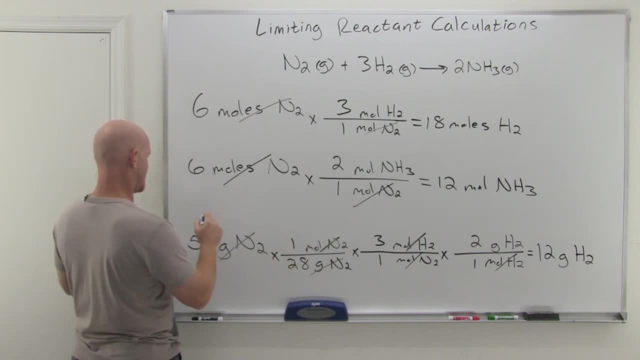 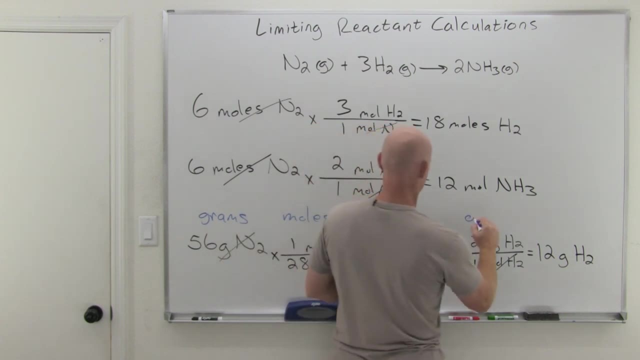 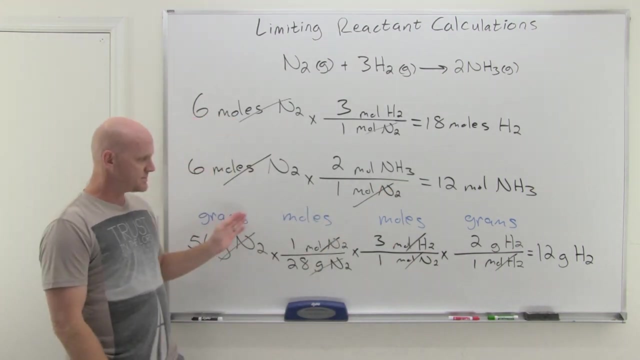 grams and you end with grams. So this is often what we refer to as your grams to moles to grams type calculation. So commonly you hear that grams to moles To moles to grams And grams to moles and moles to grams. that's always a connection through the 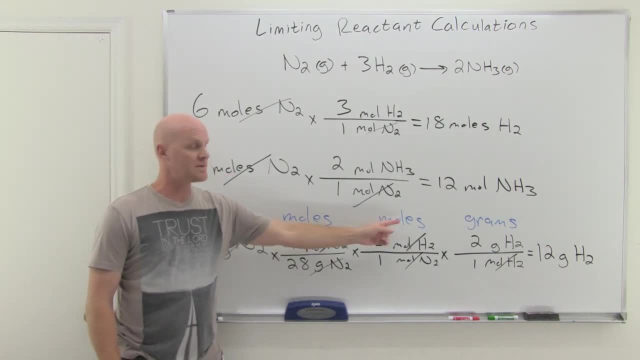 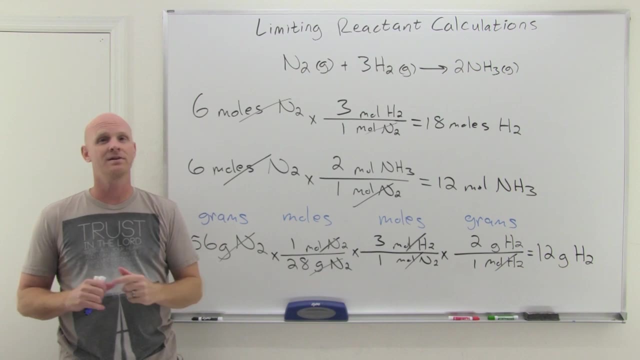 molar mass of whatever chemical species you're talking about, But it's the connection between moles and moles And that is where you're required to use a mole to mole ratio. And in this case, again, we're getting that from the coefficients in the balanced reaction. So now we're going to 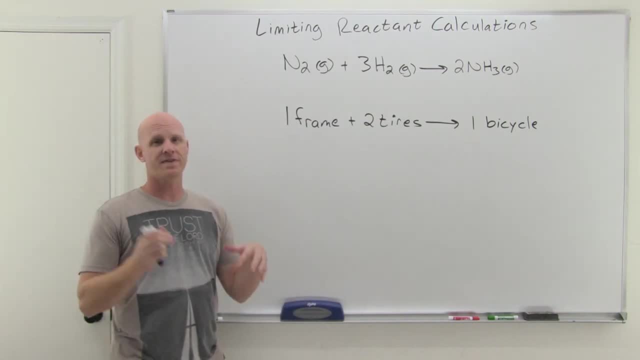 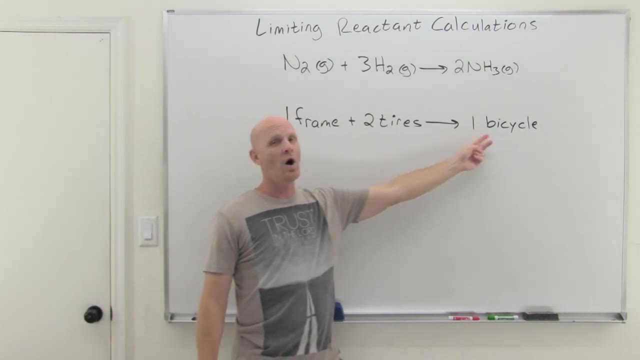 get into limiting reagent calculations a little more proper here And I'm going to come up with a mock fake chemical reaction here. that's not really chemical in nature at all. But one frame plus two tires can make one standard Bicycle here. That's what we're going to deal with, And so if I look at the ratio of frame to 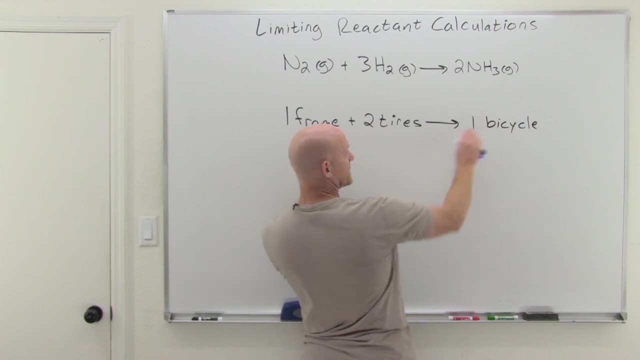 tires, it's a one to two ratio. If I look at the ratio of frames to bicycles, it's a one to one ratio. Or tires to bicycle: it's a two to one ratio. And we're going to do what's now called. 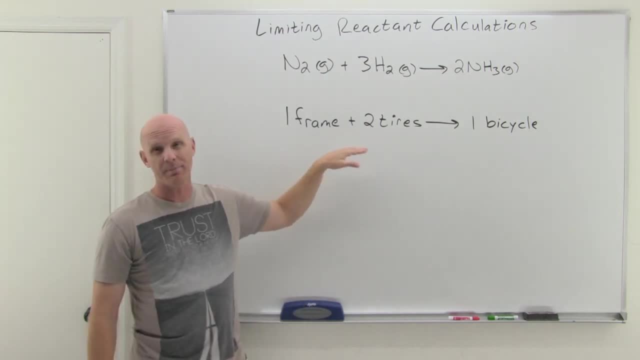 a proper limiting reactant calculation here using this example because it's something that you can see. Once we start doing this with compounds and molecules and atoms, it gets a little bit vague in students' minds and they can't picture it. But we'll do it with something we can picture. 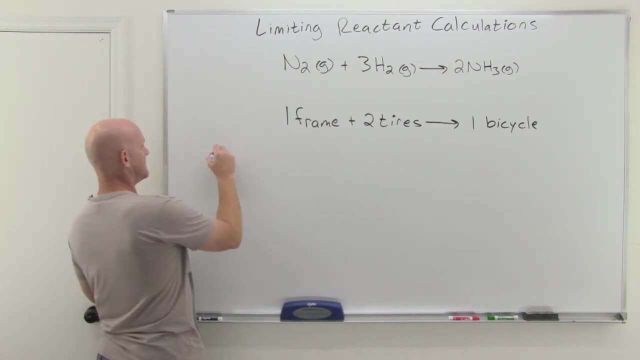 first. So let's say that I gave you 10 frames- 10 frames- And my question would be: you've got 10 bicycle frames. what number of tires do you need to use up all your frames? Well, based on the one to two ratio, you would need 20 tires, And I'm guessing there's a really good chance you're not. 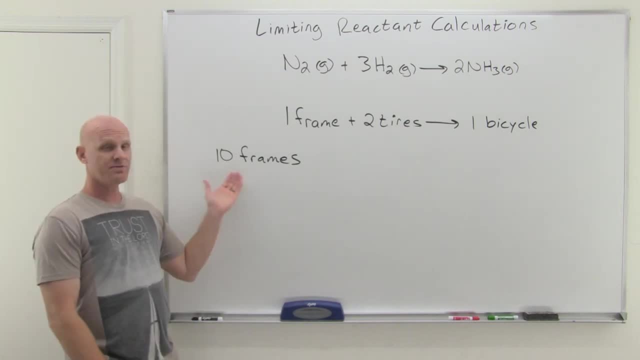 struggling to figure this out, And my next question is: if I give you 10 frames, what is the greatest number of bicycles, complete bicycles- that you could make? Well, 10.. It's based on a one to one ratio. 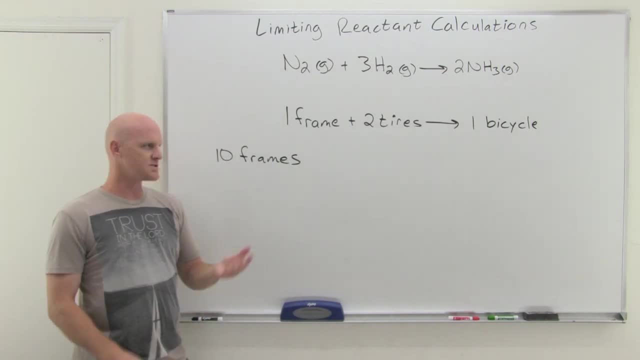 What is the greatest number of complete bicycles that you could make? Well, 10.. It's based on a one to one ratio. For every frame, you can make no more than one bicycle. So 10 frames can make 10 bicycles. 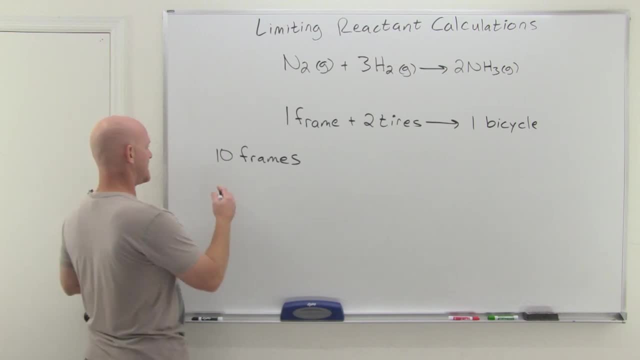 So what if I gave you 10 frames and then I gave you 22 tires, And the question is: how many bicycles can you make maximum? What's the greatest number of complete bicycles you can make? And so there's a couple of different ways to figure this out. 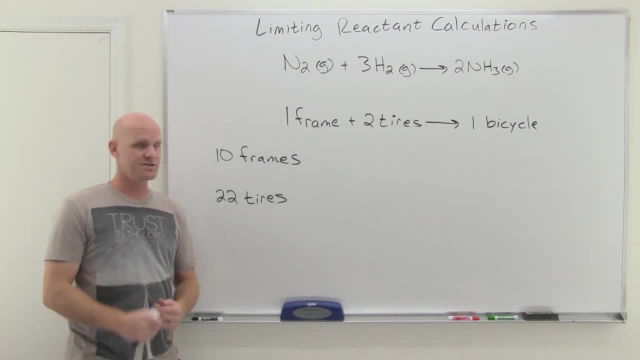 And we have to talk about what's called the limiting reactant or limiting reagent, And it's whichever one of these limits The greatest number of bicycles we can make. So whichever one's going to run out first, we might say. And so in this case again, you're probably not struggling to see this. 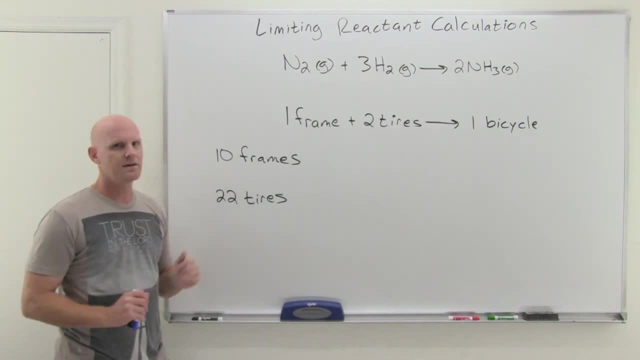 You're probably just looking at this- and be like Chad: you can make 10 bicycles, Okay, And I want it to be that intuitive for you, Because once again we start applying this to a chemical reaction stuff like that, It's going to get a little more, a little harder to see, so to speak. 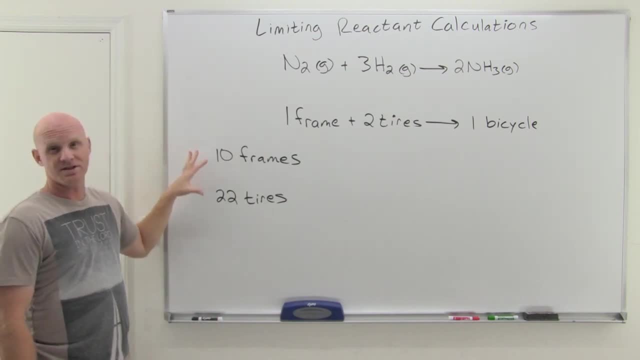 So in this case- the way I want you to approach this- and there's multiple different ways to figure this out- You could look at this and say: well, 10 frames needs 20 tires. Since I have more than 20 tires, then the 10 frames is the limiting reactant. 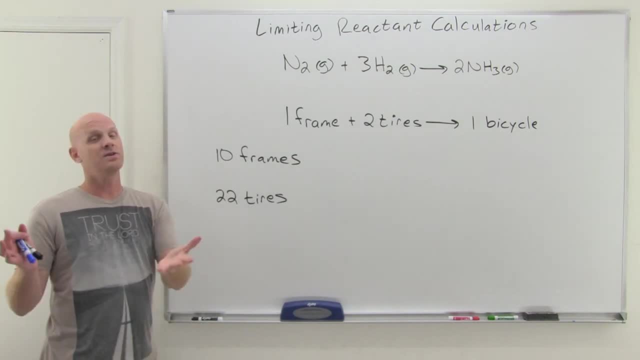 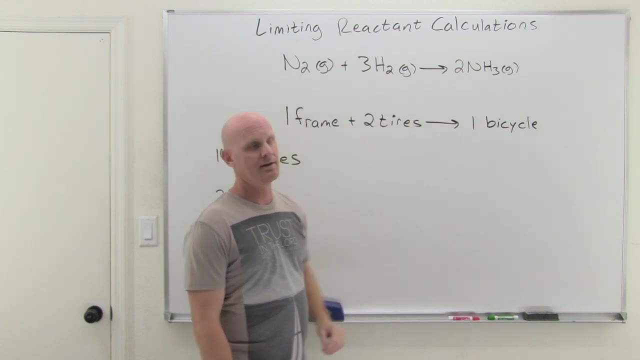 I have more than enough tires for all 10 frames to react, And you can totally do that. It's just not the approach I'm going to take. What I'm going to do is figure out how many bicycles I can make based on using up all the frames. 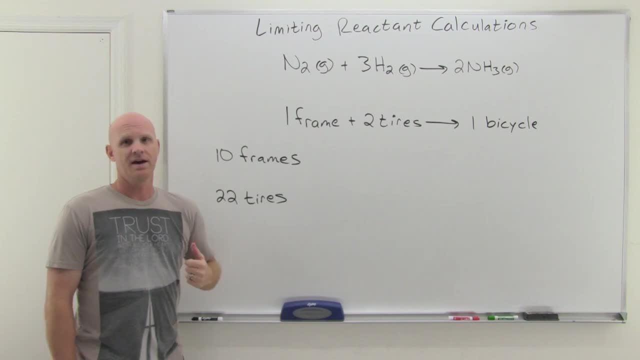 and then separately, based on using up all of the tires, And whichever one leads to a lower number of bicycles, a lower number of product. in this case, that's the limiting reagent. So in this case, 10 frames, based on the one-to-one ratio, can make me 10 bicycles. 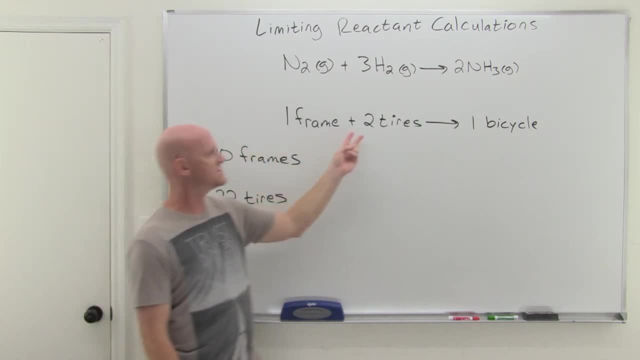 Maximum, But 22 tires, based on the two-to-one ratio, can make me half as many or 11 bicycles. So we have enough frames to make 10 bicycles. We have enough tires to make 11.. Well then, we can only make 10 bicycles. 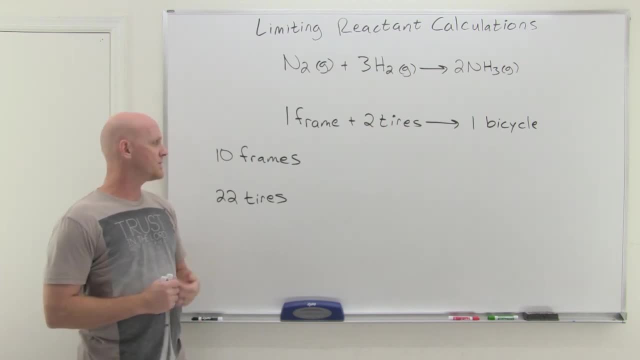 You're going to run out of frames before you've used up all your tires. So we would call the frames the limiting reactant or limiting reagent. We call the tires the reagent in excess And the fact that we can make a maximum of 10 bicycles we'd refer to that 10 bicycles. 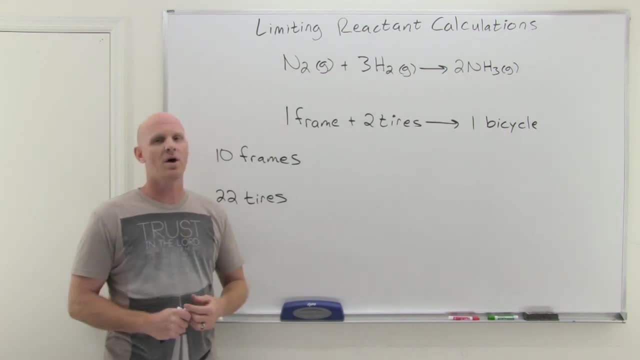 as the theoretical yield of our product in this case. So that's kind of the idea here. And again, I'm not even working this out proper. We'll work this out proper in a little bit with a real chemical reaction, But I wanted to use an example that you can see and with numbers that are nice and things of this sort. 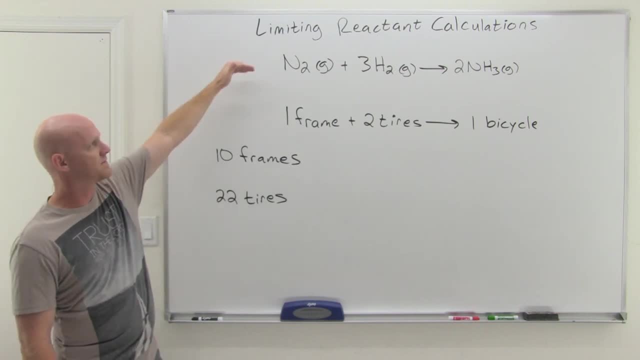 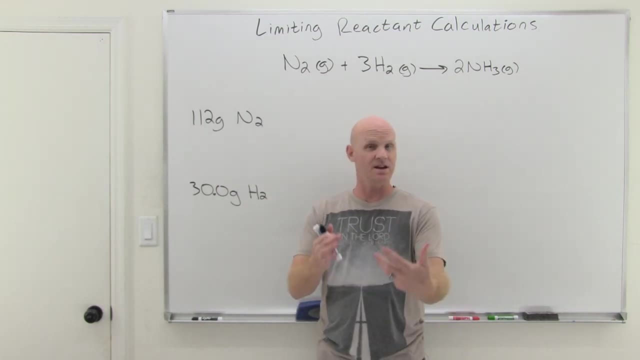 But that's kind of the approach we're going to take, And so let's see how this applies to an actual chemical reaction here. So now we're going to do a limiting reactant calculation proper, or at least a set of calculations, And in this question we're going to be given 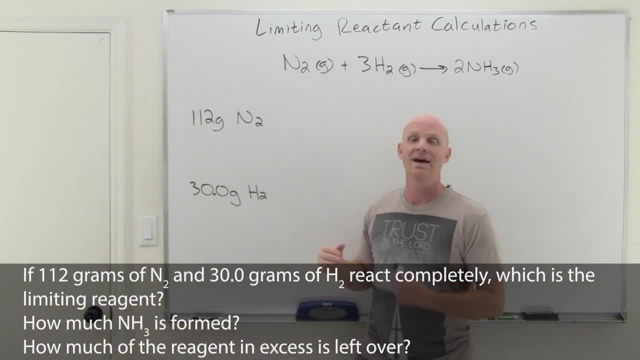 112 grams of N2 and 30.0 grams of H2.. And they are going to react completely. And we've got three questions to answer. And the first question is: what is the limiting reactant or limiting reagent? Same diff? 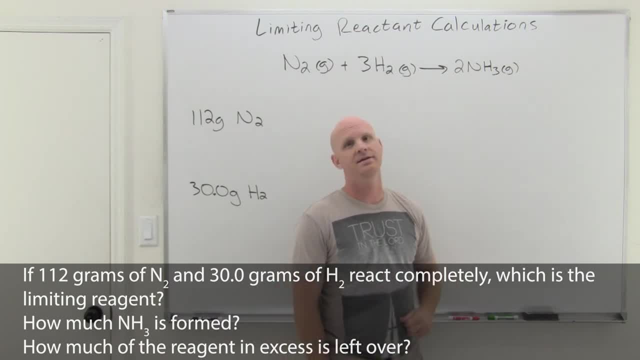 Second question is how much NH3 is formed if these do react completely. And then the last question is going to be how much of the reagent in excess is left over. All right, So the first question is: what is the limiting reactant? 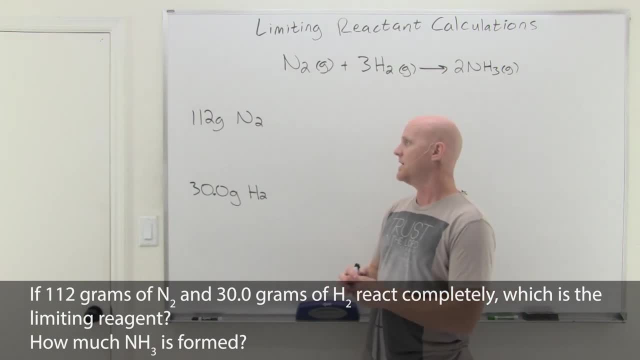 And really that's going to be the one that runs out first. Now there's a temptation here to look and be like: well, I've got 112 grams of N2 and only 30 grams of H2. So obviously I just have way less H2.. 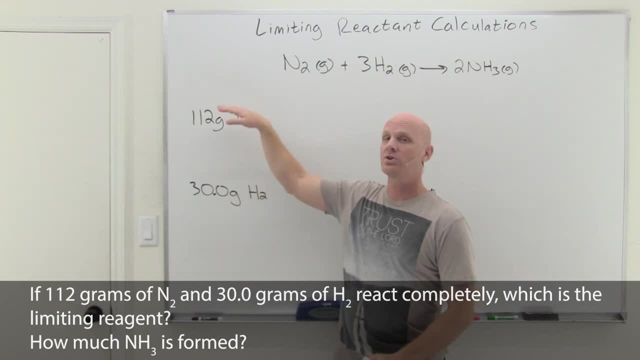 But you can't look at it that way, And so one: these are given in grams, So not moles, And I know that you know it's a one to three ratio in moles. I don't know what the ratio is in grams. 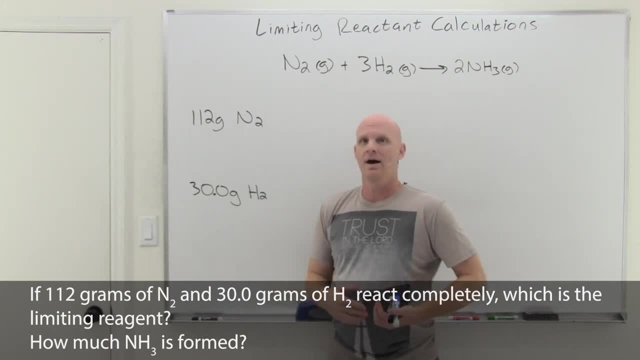 And so, first of all, it's not even a one to one ratio, It's a one to three ratio. And again, that's ratio of moles, not a ratio of grams. And so don't, don't yield to the temptation that just says: pick whichever one you have less of, because it's not usually true. 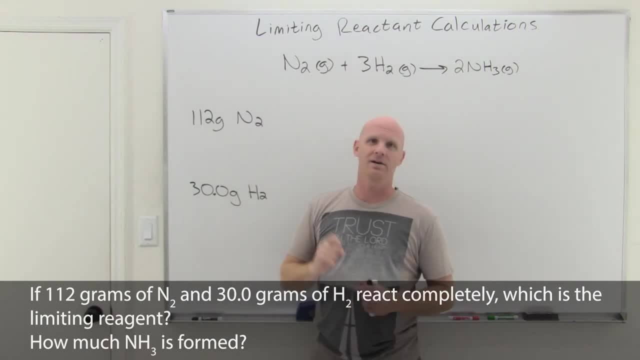 You know, randomly it could be either one. But you know a good instructor is going to write a question in such a way that if you just go with the easy temptation here to pick whichever one you have less of as limiting reactant, 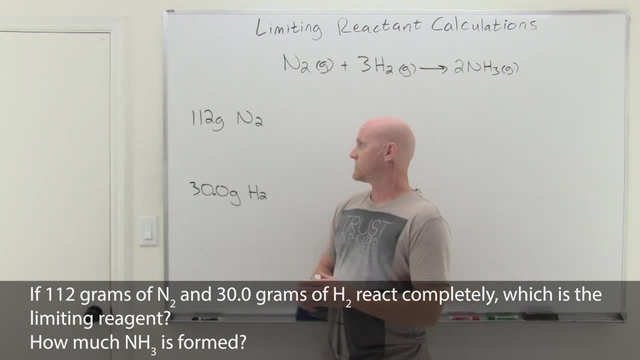 it's probably going to be wrong. So just word of the wise, All right. So what we need to do is figure out how much NH3 we can make maximum if either one of these runs out, And again, whichever one leads to less is going to be the limiting reactant. 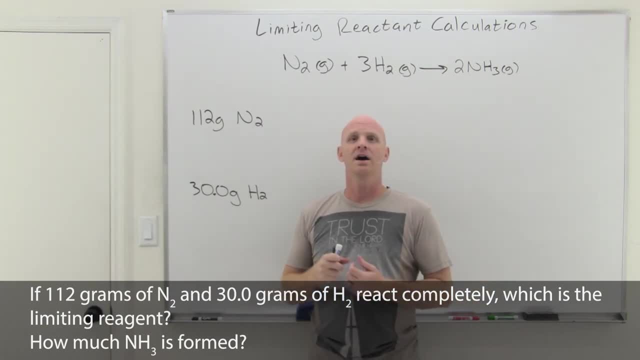 It's kind of like if I was into construction and I have enough bricks to make a thousand homes. I build homes. let's say So: I have enough bricks. I have enough bricks to make a thousand homes, But I have enough drywall to make three homes. 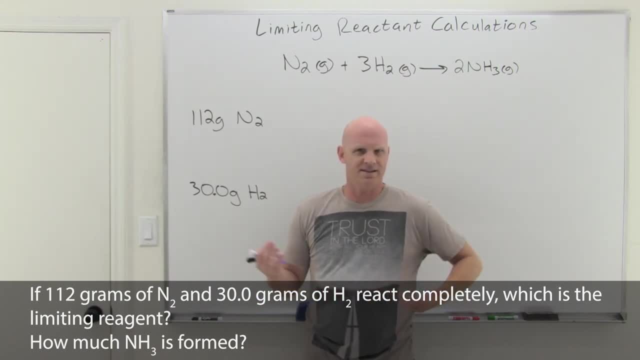 So can I make a thousand homes or can I make three homes? Well, obviously, with the supplies that I have on hand, I can only make three homes, and I'm out of drywall. Drywall would be the limiting reactant in that case. 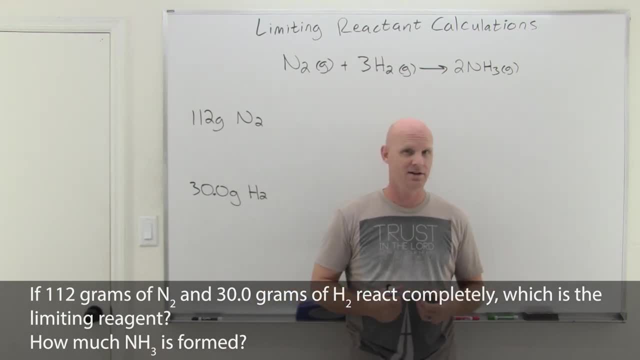 And the bricks would be the reagent or reactant in excess. That's kind of how that works. So we're going to figure out how much NH3 we can make, assuming either one of these runs out completely, And whichever one makes less is the limiting reactant. 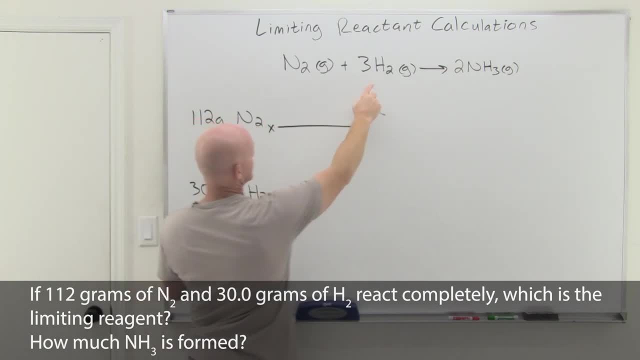 All right, So we're going to convert this to moles. I can relate the moles of N2 to NH3 based on this one mole to two mole ratio, But I've got to have moles, And so the first thing we're going to do is just turn this into moles. 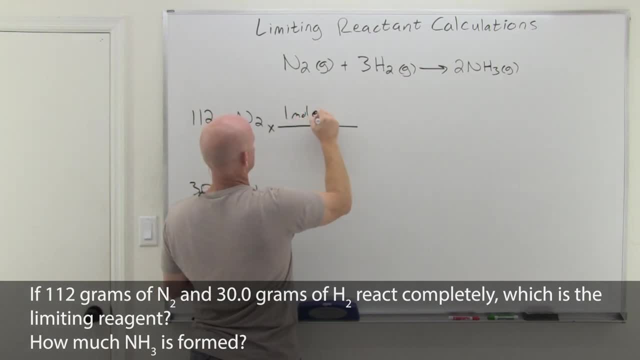 And so in this case, one mole of N2 weighs 28 grams. Again, it's diatomic, And now that I've got the moles of N2 here, we can then convert that into the moles of ammonia, NH3, from N2.. 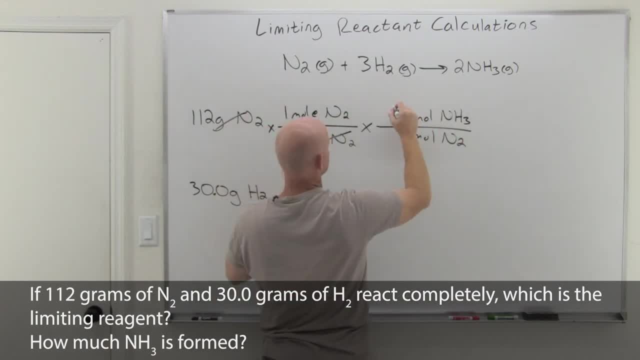 And that's that mole to mole ratio, Which in this case is just the coefficients in the balanced reaction. So that's a two to one ratio And we'll go from there. So 112 divided by 28 is exactly four, it turns out. 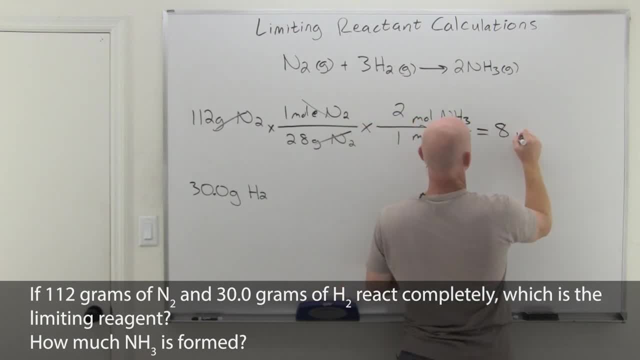 And four times two over one is eight, And so if all of our N2 reacts completely, we would get eight moles of NH3.. Now hydrogen is going to be a little easier on the math here, But again, we've got to convert this to moles first. 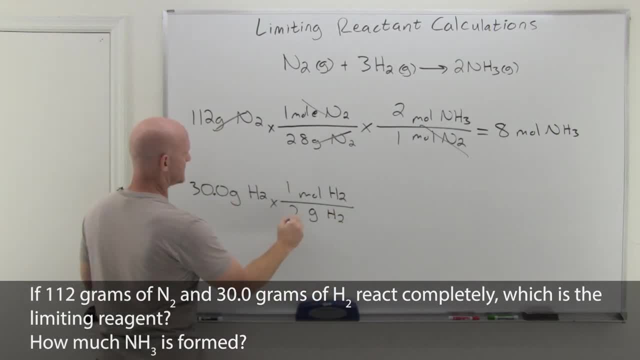 So- and again that's through molar mass. One mole of H2 weighs two grams, And so 30 grams is going to end up being 15 moles, And we can kind of see that we've got a three to two mole to mole ratio. 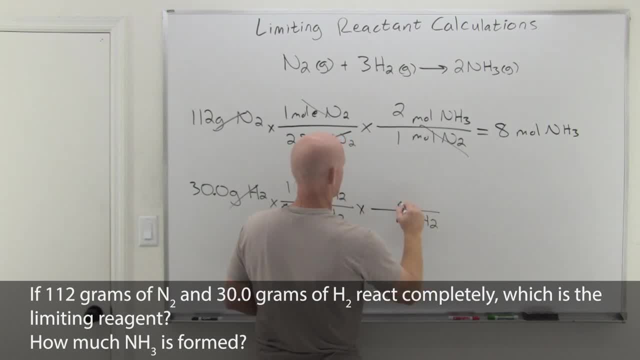 We'll put moles of H2 in the denominator, Moles of NH3 in the numerator, And again it's just the coefficients right out of the balanced reaction. So two moles to three mole ratio, And so in this case, 30 divided by two is 15.. 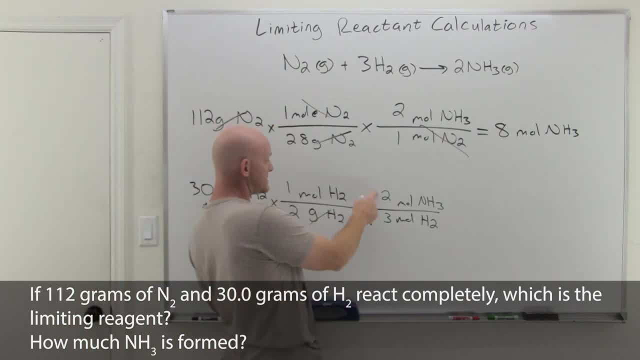 And 15 divided by two thirds, Or say 15 multiplied by two over three, Multiply by two thirds is equal to 10 moles of NH3. And so you're supposed to take this, now that you have enough N2, to make eight moles of NH3. 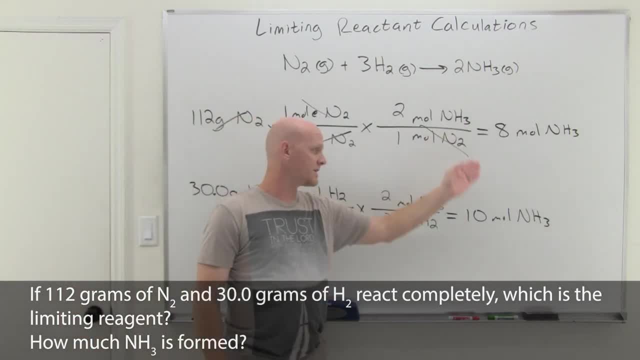 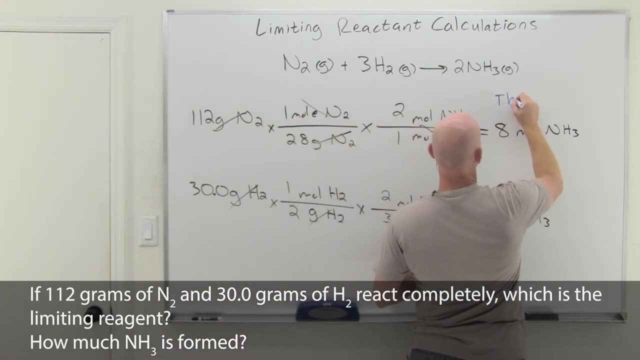 You've got enough H2 to make 10 moles. So can you make eight moles, or can you make 10 moles? Well, you can only make eight moles. That's kind of the idea here, And we call this eight moles. here the theoretical yield, 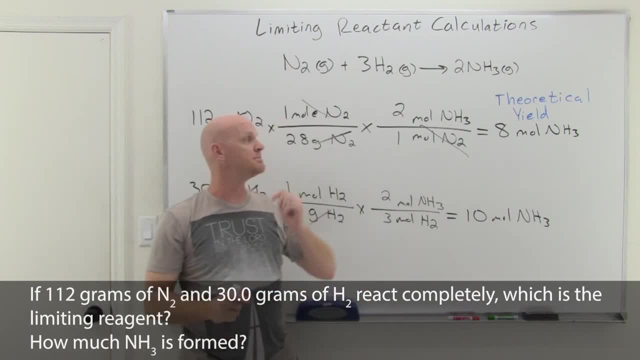 It is the maximum number, That's the number of moles of NH3 we could possibly make, And the reason we call it the theoretical yield is because usually you don't make the maximum. It turns out that for most chemical reactions there are certain side reactions that are sometimes possible. 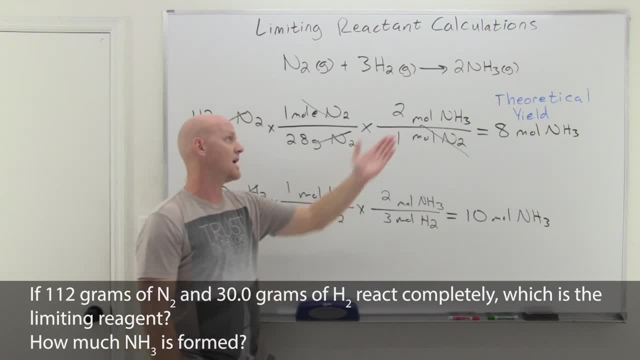 And so some of the reactions get used up in making these other side products and not making the product of interest. So you never end up getting this maximum. We'll also find out that most reactions don't go to completion, But you'll find that out in your second semester. 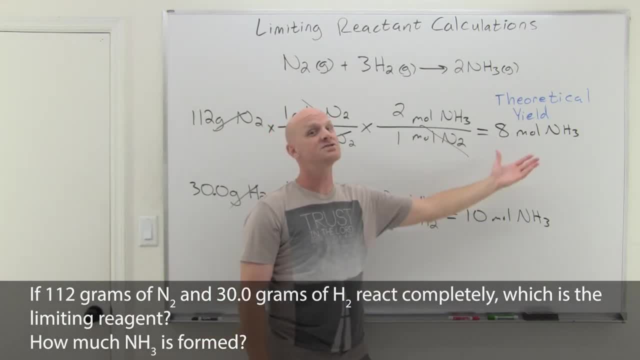 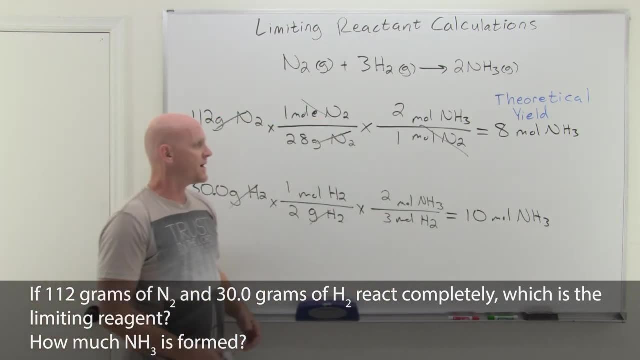 But it just turns out this is what we call the theoretical yield. Theoretically, this is the most you could ever get, even though in practice we usually don't even get this much. All right, So there's our theoretical yield of eight moles. 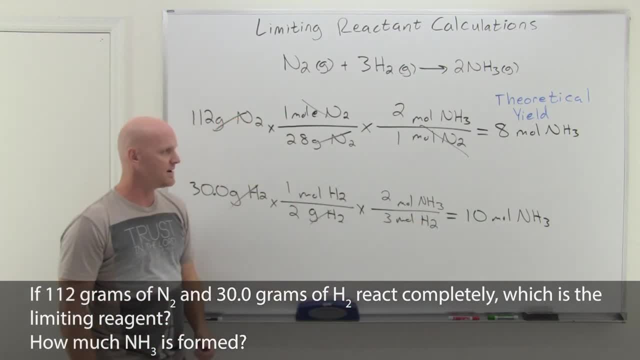 We're never going to have any chance of getting 10 moles. We just don't have enough N2 to get there. And so now we've answered two questions: Our limiting reagent here or limiting reactant? same diff is N2.. 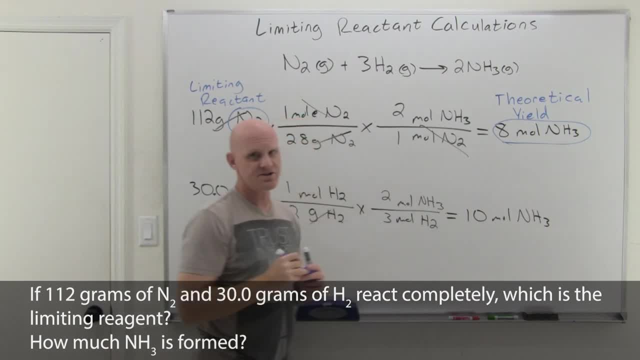 Our theoretical yield here is going to be this: eight moles, Eight moles of NH3.. So in this methodology, we've actually solved for both at the same time. Now, if you were doing this as a multiple-choice test question and if they asked you what's the theoretical yield, 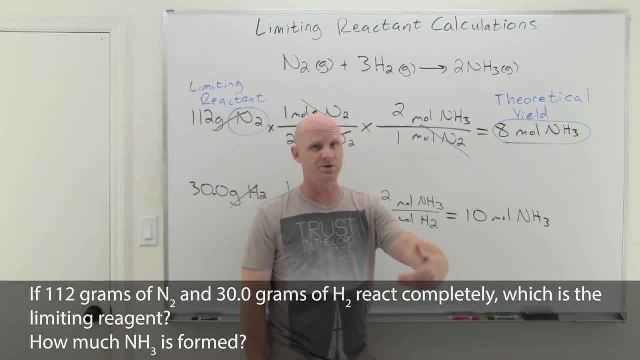 Or, as I asked it, what is the greatest number of moles of NH3 that could be formed or produced, or something like this? They could ask this in moles or grams, And had we asked this in grams and all the answer choices in a multiple-choice question, but in grams, you would have had to have taken this one step further. 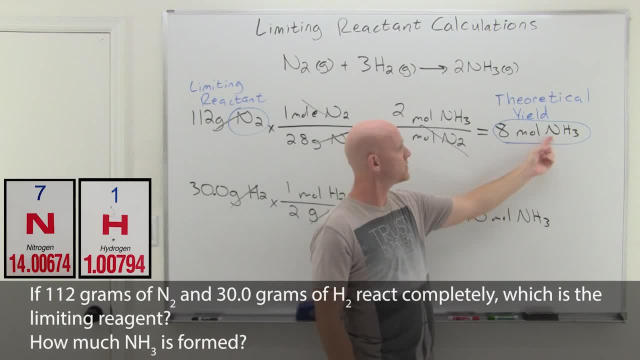 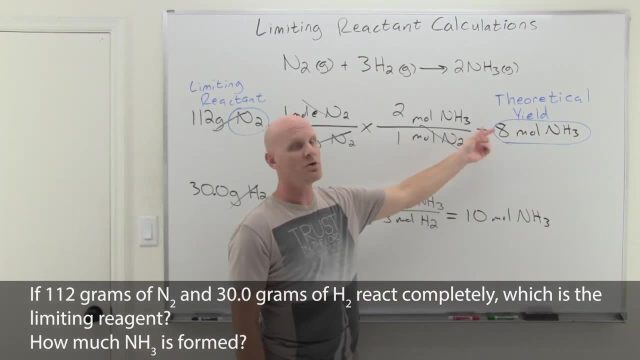 And you'd have to figure out that the molar mass of NH3 is 17.. So 14 plus 1 each for those three hydrants. So 14 plus 3 is 17 grams per mole, And you would have multiplied 8 times 17,, which would have given you like 136 grams of NH3. 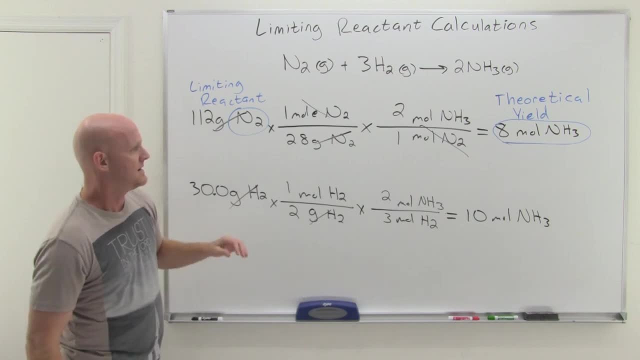 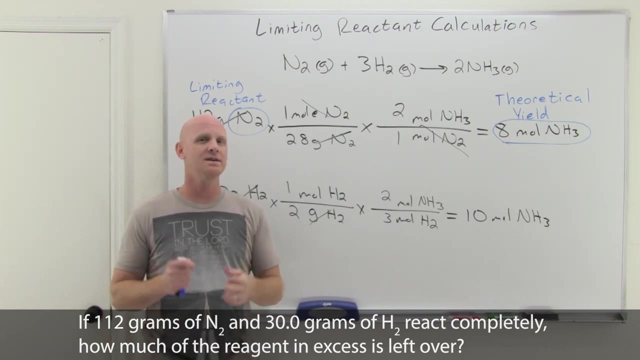 But I'm going to stop there. That was sufficient for what I was asking, And the next question, though, is the last one here in the assignment, And it's the most challenging one for students, And the question is how much of the reagent in excess is left over. 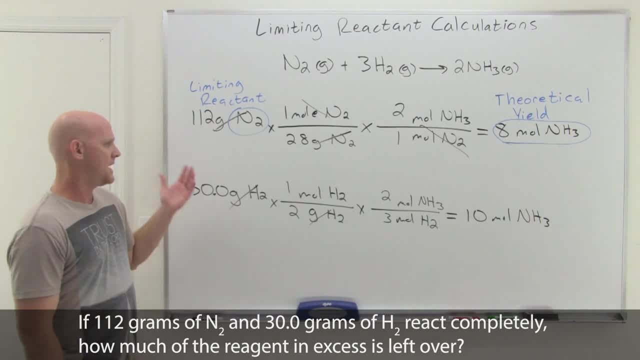 And that could be how many moles or how many grams, And we'll do both- And in this case, we can see that the H2 is the reagent in excess, And the question, though, is how much is left over. 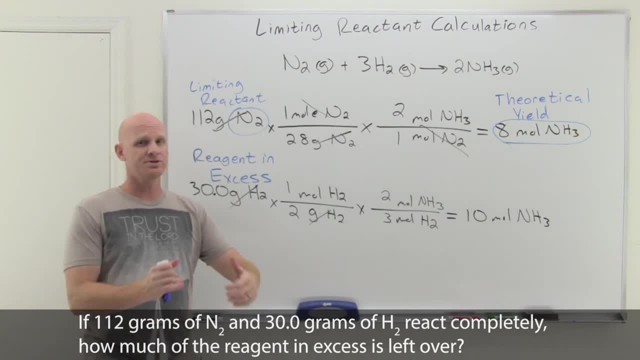 And when you're going to figure this out, you want to start from a theoretical yield you just calculated And the idea is that you know how much of this H2 that you have, that you've started with. The question is how much actually gets used up in making your theoretical yield of your product. 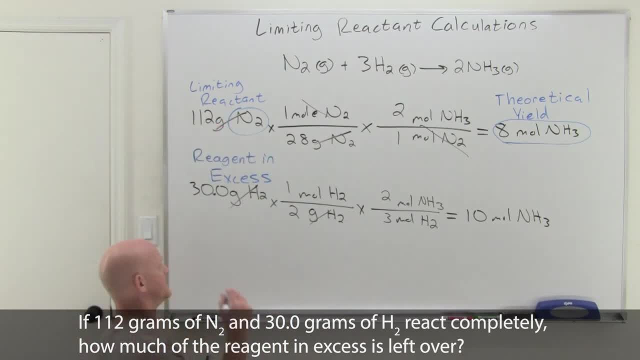 And then we'll just subtract that off from how much we started with. So we're going to start with that theoretical yield of 8 moles NH3. And I want to find out how much of the H2 got used up. So we'll relate the moles of NH3 to the moles of H2.. 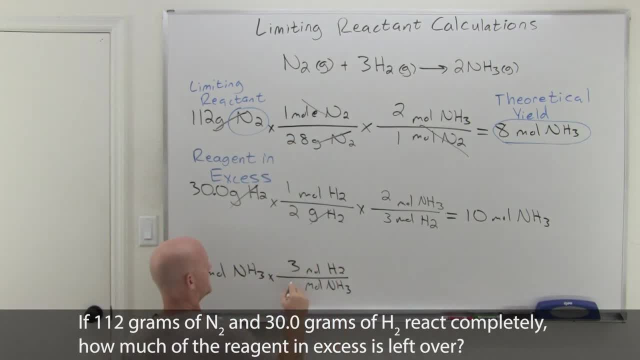 And that mole-to-mole ratio once again comes from the coefficient, So 3 moles of H2 for every 2 moles of NH3. And we'll take this one step further and go to grams. here And again, that connection between moles of H2 and grams of H2 is always the molar mass. 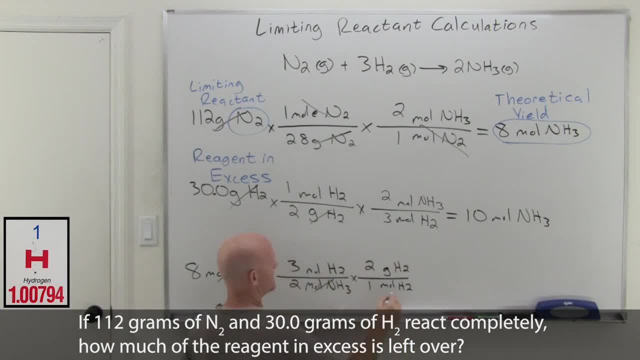 And 1 mole of H2 weighs 2 grams, And then 8 times 3 halves, And then this 2 will cancel right here. So 8 times 3 effectively is 24 grams of H2.. And this is how much is going to be used or consumed. 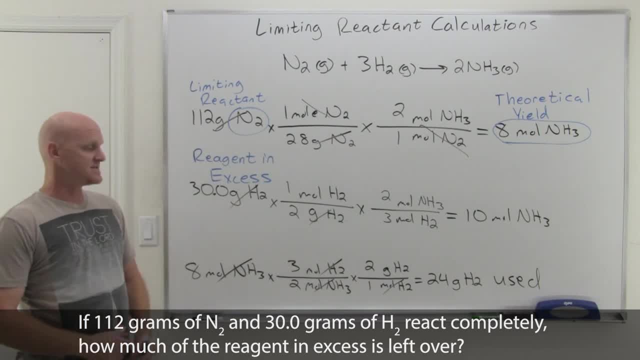 And so we started with H2.. We started with 30 grams. We just figured out that, to get our theoretical yield of 8 moles of ammonia, that 24 of those grams are going to get used up, And so we'll just subtract that off. 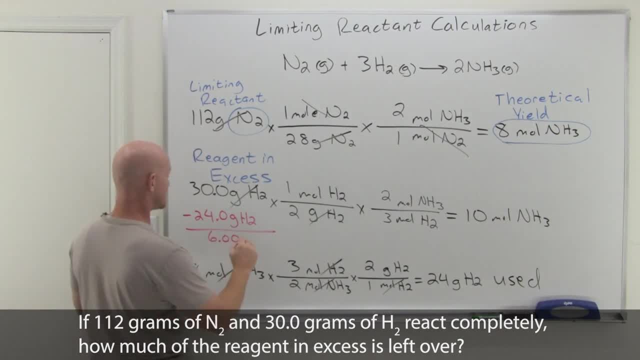 And we'll see that we've got 6.. And to get 3 sig figs, we'll make it 6.00 grams of H2, either left over or in excess is the way we might say that Cool. And the big mistake that a lot of students make is they'll sometimes figure out. 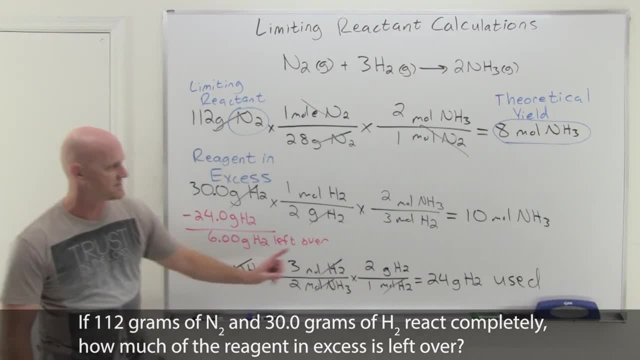 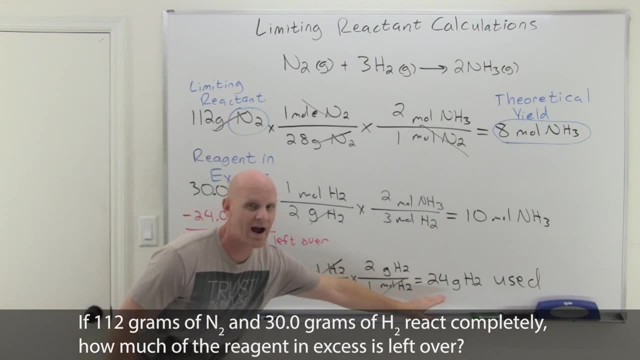 that they need to start with this theoretical yield, But then they think that they just calculate directly to here when again they're going to take the original amount of the reagent in excess they started with and subtract off how much actually was used that we calculated here to get that difference. 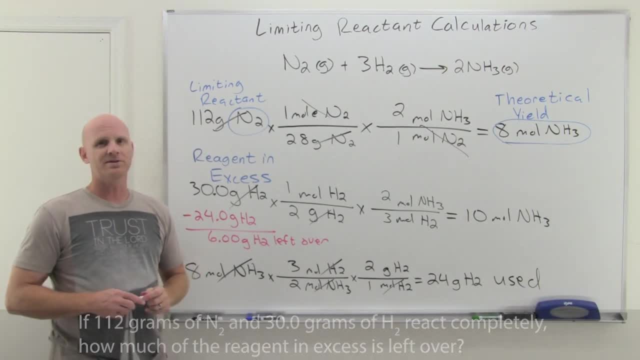 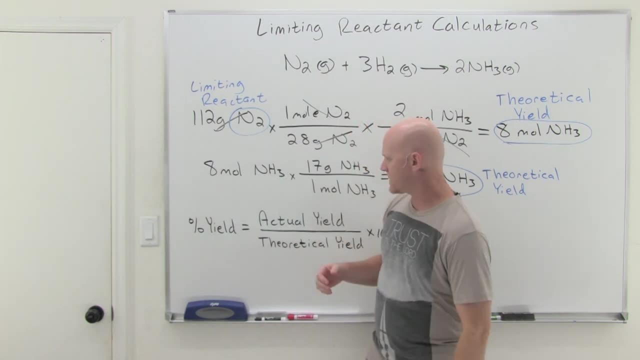 And it's that difference, that is the amount that's left over. All right, So we've got one last little calculation to do, And that is a percent yield calculation. And it turns out your percent yield is equal to what's referred to as your actual yield. 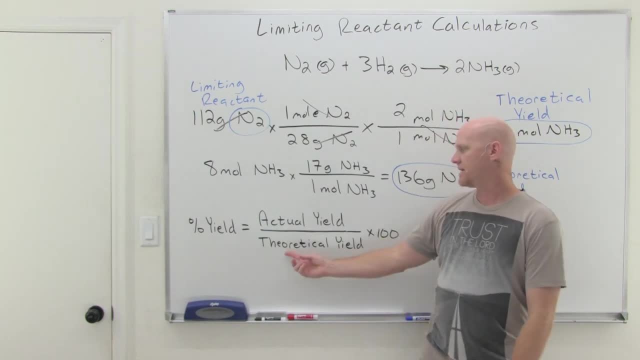 how much product you actually got divided by your theoretical yield times 100.. And, if you recall, we said that your theoretical yield is theoretical in the sense that you know you might have some side reactions happening that use up some of your reactants. 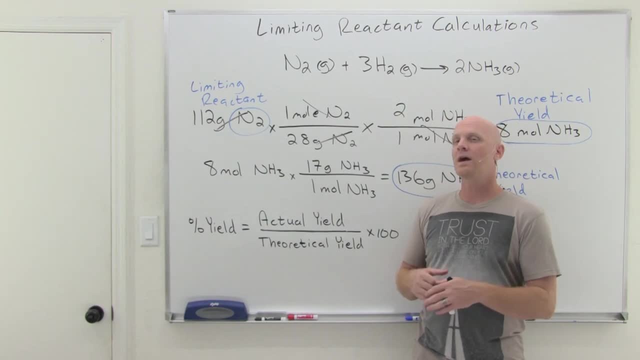 and so not all your reactants end up going to make products and that most chemical reactions don't actually go to completion. So for a lot of times you'll end up with leftover reactants and not making as much product as you did. 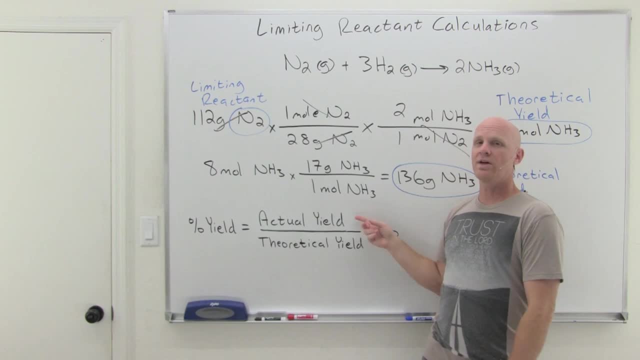 And so that's why it's convenient to talk about this actual yield, how much you actually got. And again, it should be less than your theoretical yield. You know for a lot of organic chemistry students they'll end up with an actual yield. 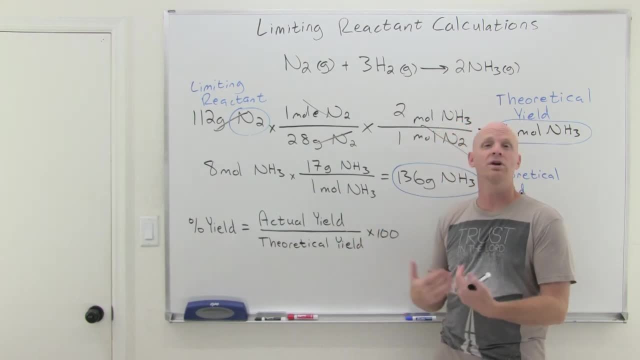 That's bigger than their theoretical yield And they'll end up with a percent yield that's over 100%, And usually that's a dead giveaway that your product is wet and you need to dry it off better, because you shouldn't be able to get more than a 100% yield. 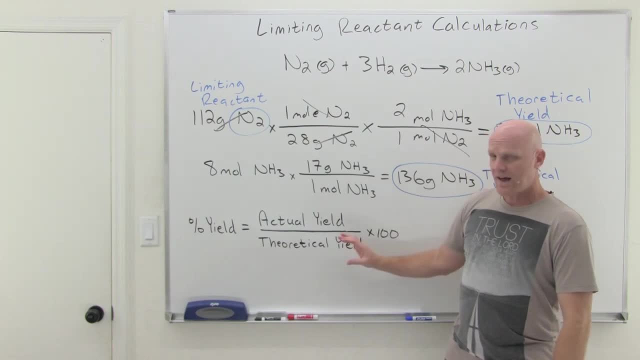 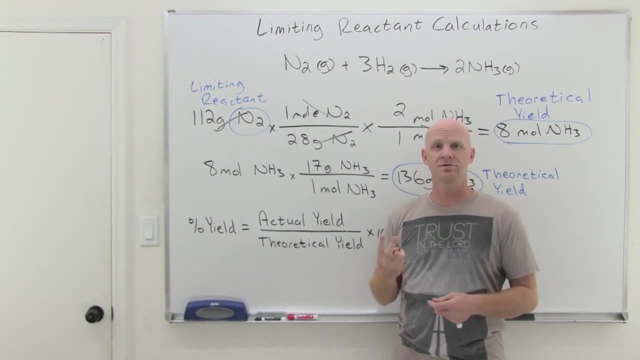 So that's kind of the idea here. So this is our last calculation And you can treat this as kind of being an equation with three variables. There's percent yield, actual yield, theoretical yield, And if you're given two of the three, you can solve for the third. 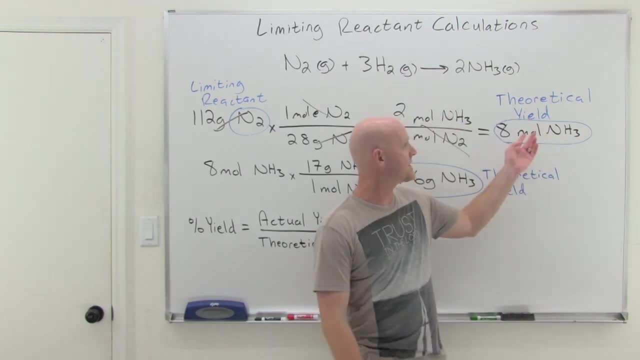 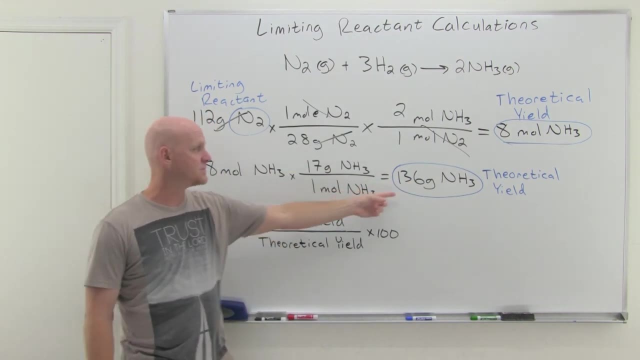 And so what we're going to do is we're going to take the problem we just did, where we got a theoretical yield of 8 moles And, if you recall, we hinted that theoretical yield if we calculated it to grams by multiplying by the molar mass. 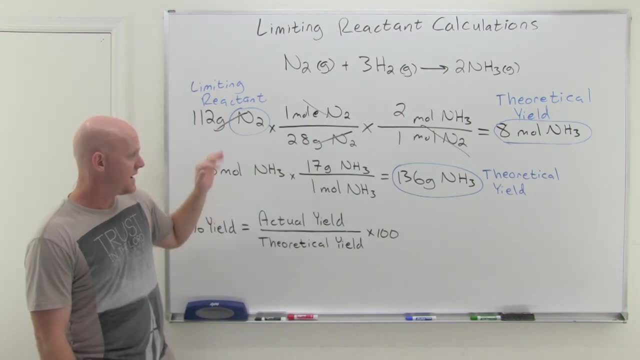 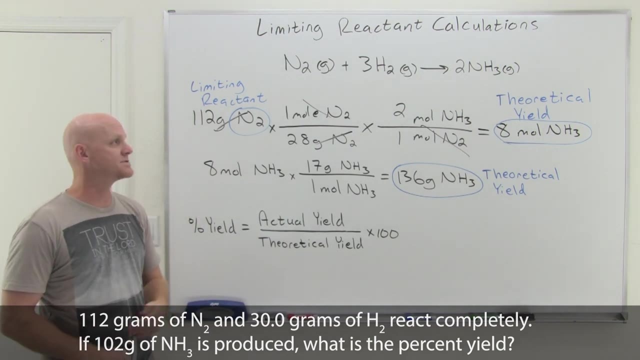 it would be 136 grams, And here I've written it out explicitly. And so we want to now say: last question on the sheet there is: if we actually only get 102 grams of ammonia as product, then what is the percent yield? So again, theoretically we see that we could get 136 grams maximum. 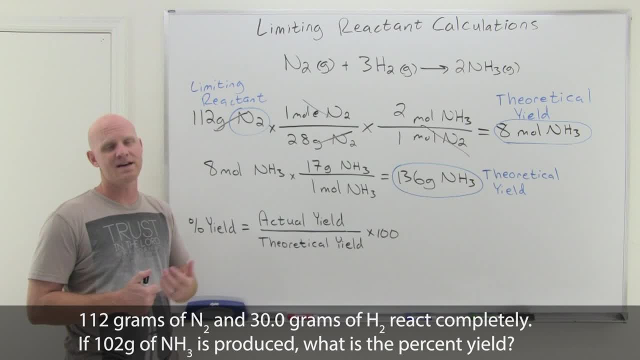 Well, we only got 102 grams. So what percent yield is that? And you can kind of think of this like, let's say I gave you enough money to go buy 10 pizzas And you only come back with 8 pizzas. 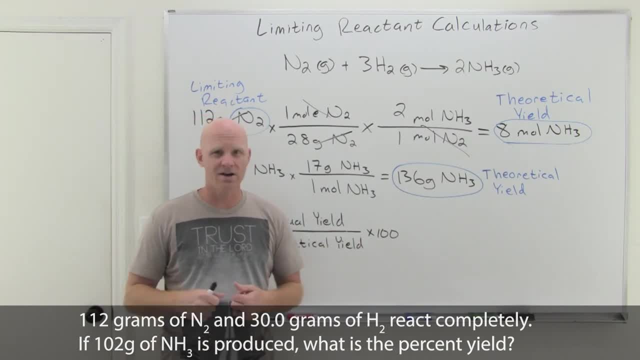 And I'm like: where's the other two pizzas? And you just pocketed the cash or something, So you only came back with 80% of what I sent you out for. That's an 80% yield: 8 out of 10 possible pizzas. 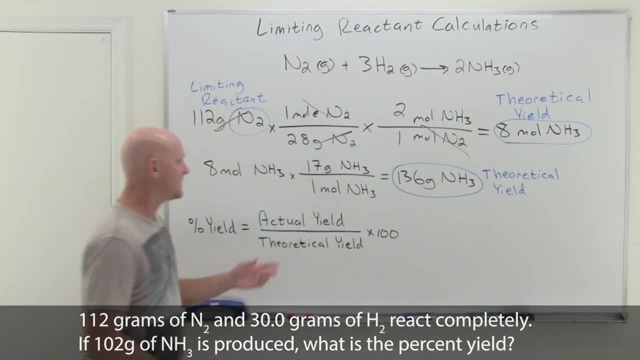 So kind of the way it works here. So with this theoretical yield calculation, we'll take our actual yield, again given in this question, as 102 grams, divided by your theoretical yield, which is 136 grams, And then multiply by 100. 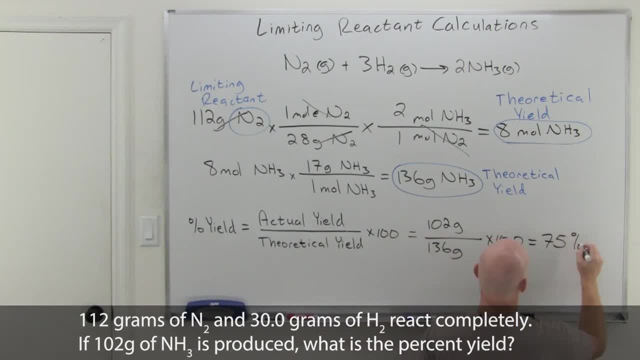 And it turns out this comes out to exactly 75%. There's your percent yield in this calculation, And you can do this in grams or moles. I just decided to put it in grams because that's most likely how you're going to see it. 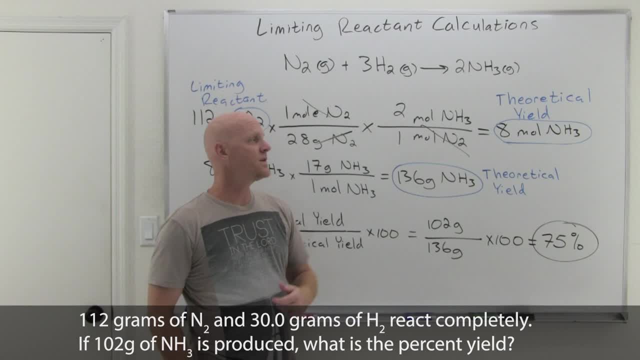 But instead of giving you the 102 grams, I could have just said: hey, you only came back and actually produced 6 moles of NH3.. Well, 6 moles out of a theoretical yield of 8,, 6 over 8 times 100 would have given you that same 75% number. 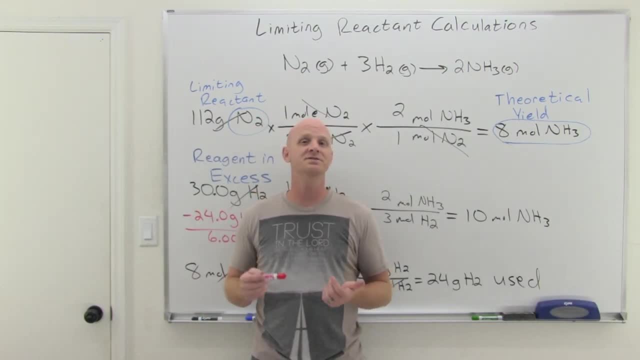 If you found this lesson helpful, a like and a share. Make sure YouTube shares this lesson with other students as well. And if you're looking for practice problems on stoichiometry and limiting reactant calculations, check out my general chemistry master course at chadsprepcom.